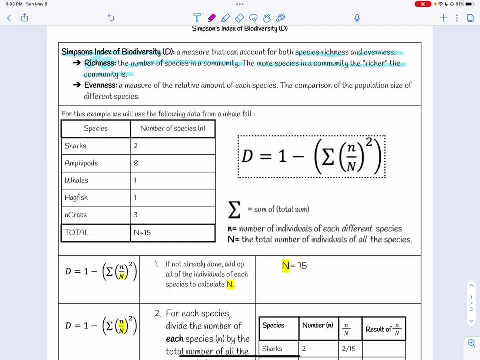 the more species in a community, the richer the community is. Remember, a community is all of the populations in a habitat or in an area. at the same time. We would say it's all the biotic factors. This also takes into account species evenness. Evenness is going to be like the relative amount or distribution, the abundance of each species. 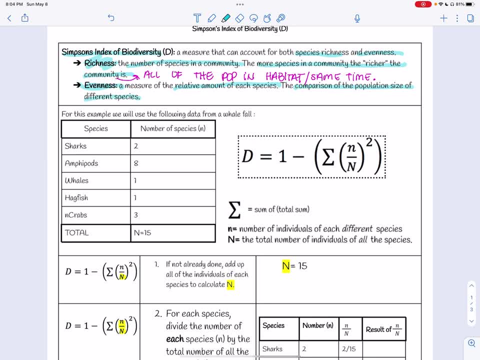 So we can compare population sizes of different species. We wouldn't say an area has evenness. if you know you have 2,000, you know seagrasses and then just you know five, just five, like sea turtles there or something. 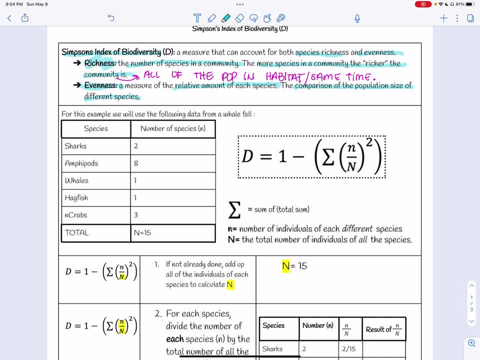 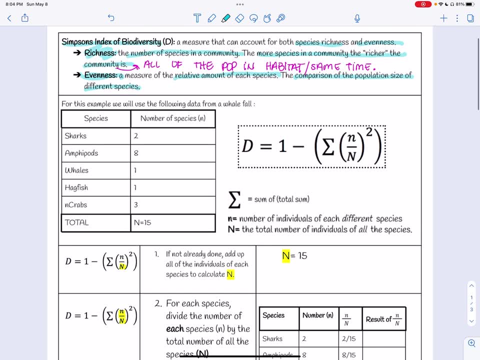 It would be comparing, you know, 2,000 within one species to five. That's not very even at all. So we're going to use this data set from a whale fall. We're going to use this data set from a whale fall. 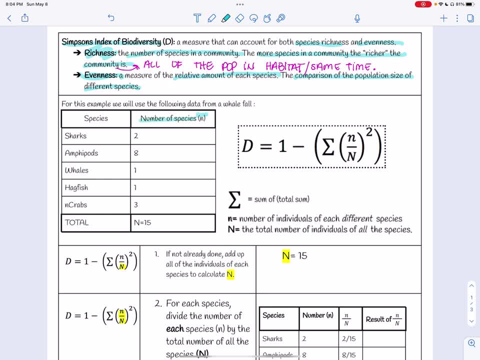 So we're going to use this data set from a whale fall Where you have the number of species, which is letter N. Oops, that one Little letter N, And for sharks we have two amphipods, or eight whales: one, hagfish one and then crabs one. 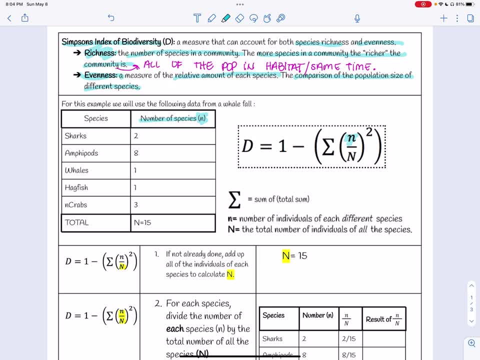 Obviously, whales will be one, because it's a whale fall. So you got one dead whale there. The total of all of your species, or all of the organisms in each species, or the total of your population, Or the total of your population- Another way to say it- is going to be big N. 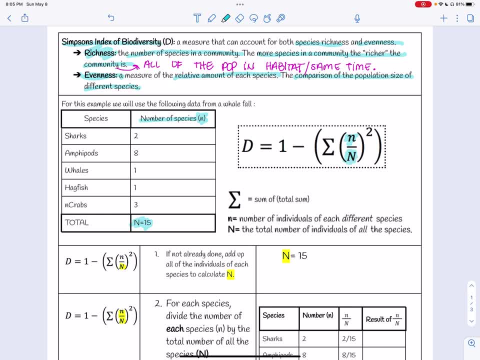 So little N is the amount in each species and then big N is the total. Again we have the summation symbol, which is capital letter S. in the Greek alphabet, Little letter S looked like this: And then your givens: little N and then big N. 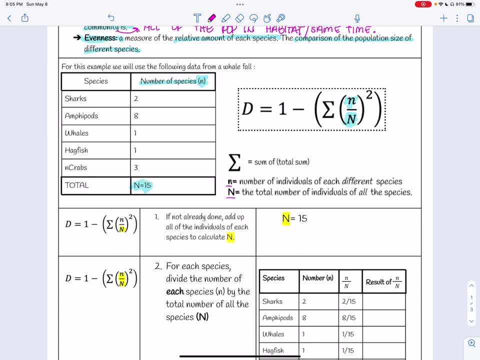 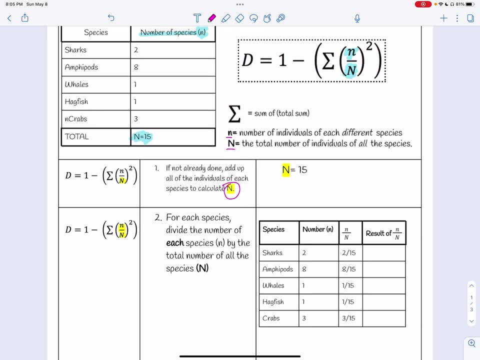 First step, if not already done: Add up all the individuals to calculate big N. So big N is 15.. Step two: for each species, divide the number of each species, which is N, So the amount in each population, by the total number of all of the species. 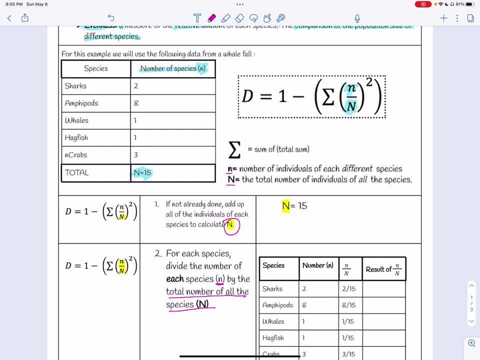 So you're going to take, for sharks, you're going to do two and you're going to divide it by 15.. For amphipods, eight divided by 15. Whales, one over 15.. Hagfish, one over 15.. 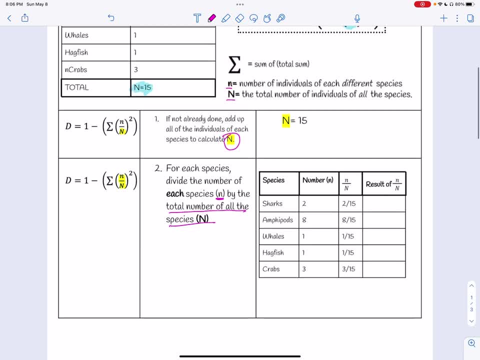 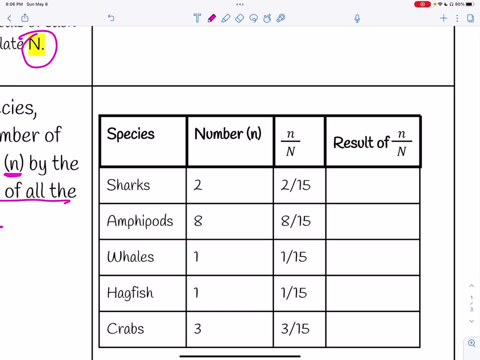 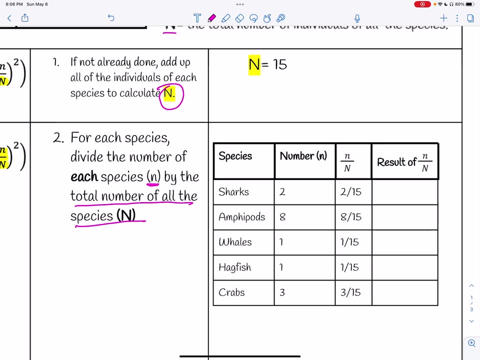 And crabs three over 15.. So it'll look something like this: So you're dividing the amount in each species by the total amount there, anyways, All right, And then we're going to put that in our results there. And this is another one where I just keep adding the same data set to each different step. 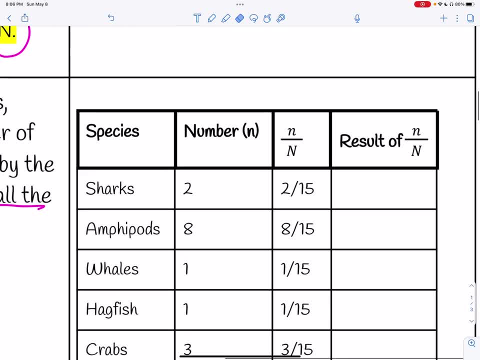 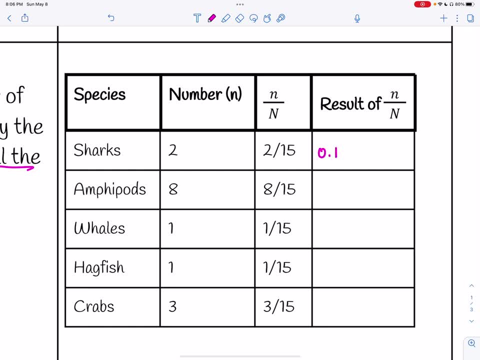 And then we're filling it in as we go. But you would just be given one data set and a question. All right, So if you divide two by 18, you'll get 0.133.. But eight divided by 15, 0.533.. 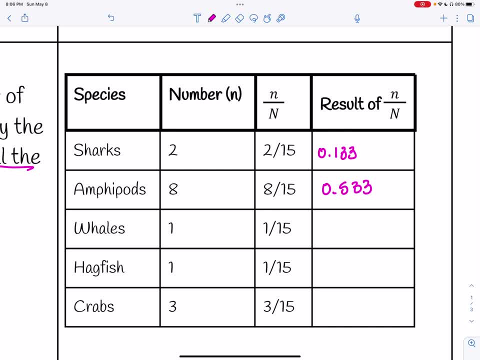 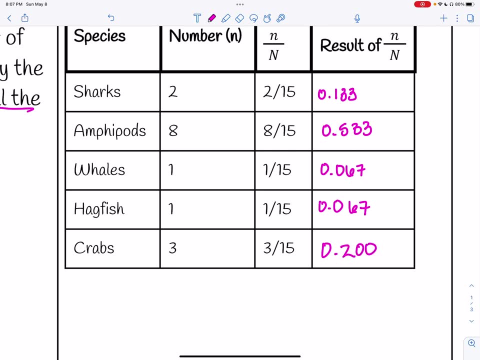 One over 15,, same for the whales and the hagfish: 0.067. And then the crabs. three over 15, 0.200. And 0.2 would be fine, but if we're just going to keep it to the thousands place, 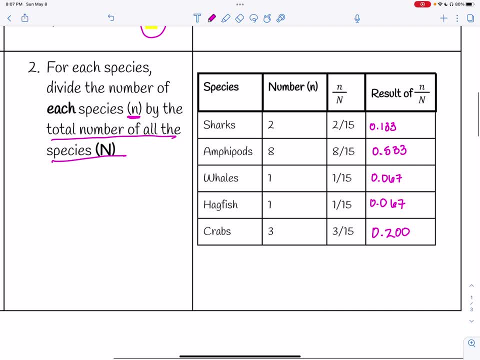 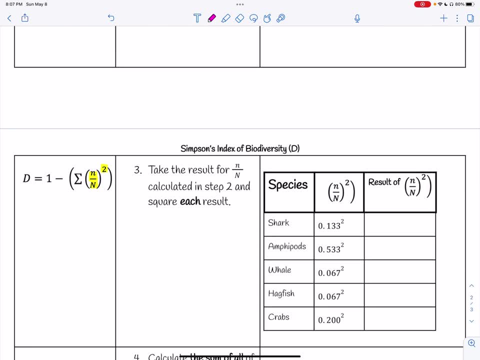 or like to three significant digits, although that's not even three significant digits. Anyway, step two's done, All right. Now we are going to be looking at the n over big N squared, So the amount in each species divided by all of the organisms there in that community. 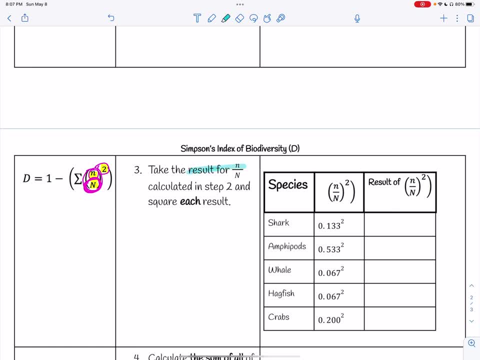 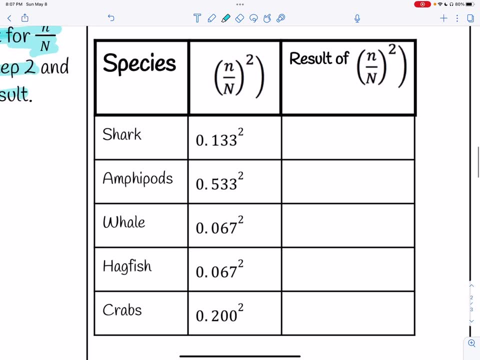 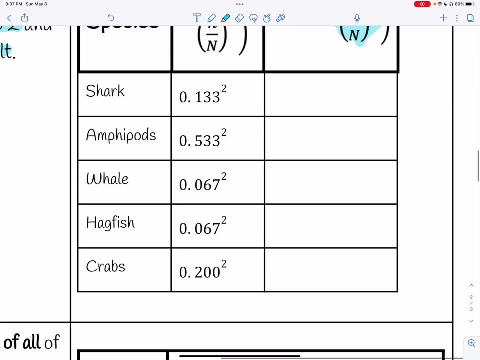 And then we're going to square it. So take the result from little n over big N from step two, and then square each result. So there's that result we're looking for 0.133 squared 0.018.. For the amphipods: 0.533 squared 0.284.. 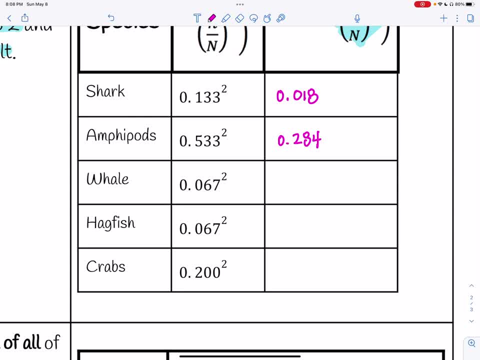 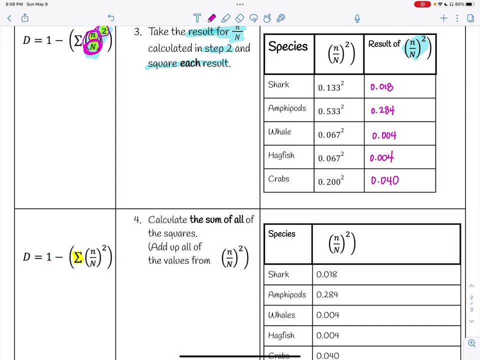 The whale and the hagfish will have the same value: 0.067 squared is 0.004.. And then your crabs: 0.2 squared 0.040.. Next step: we got the summation, So calculate the sum of all. 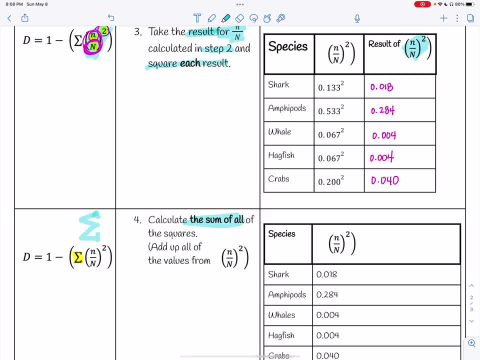 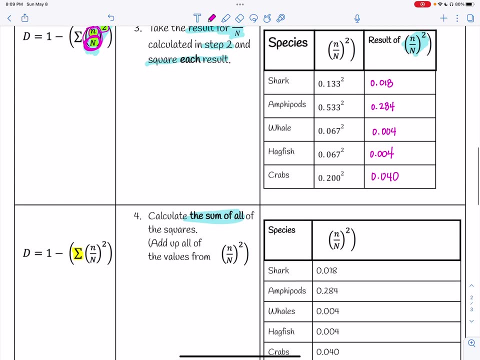 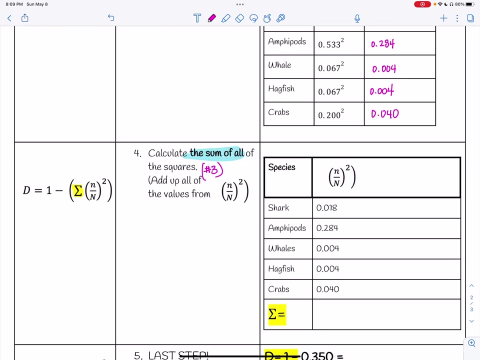 Again, that's capital letter S in the Greek alphabet sigma And this was a lowercase s. All right, Add up all the squares or all of the values that you just did from number three. If you add all those up, you're going to get 0.350.. 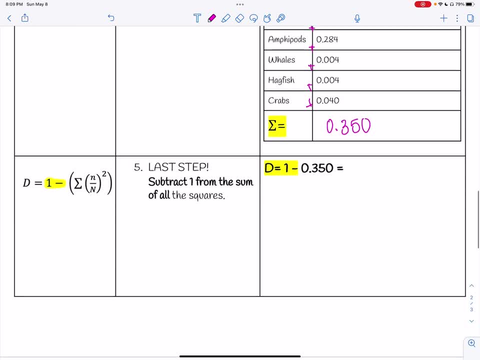 Last step is the one minus that, And you don't have to remember these formulas, You don't have to remember the variables, You just need to be able to follow the order of operations and be able to execute it. So one minus that will have 0.650. 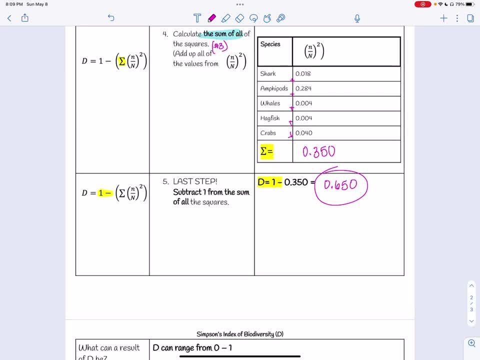 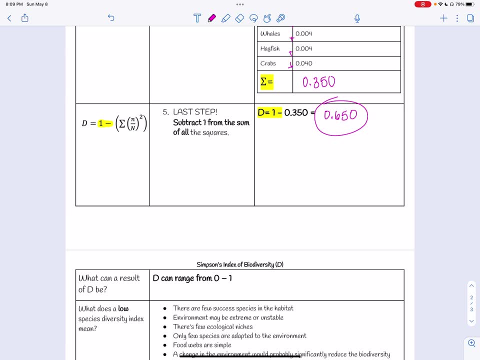 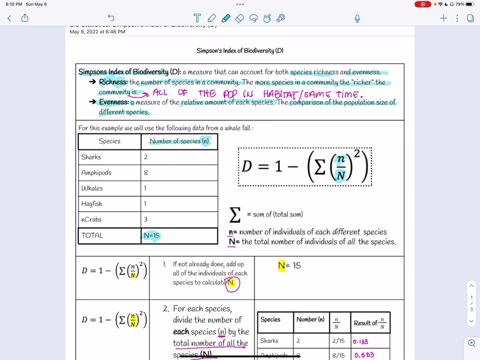 All right. So just to identify what these values can mean. And again, this is looking over the richness, so the amount of different species, And in this example we had five different species there- And then it's evenness how even they are. And even just looking at it, no, these numbers aren't large at all, But there isn't one that really dominates another. You have one massive food source, the whale One hagfish. And hagfish are nasty, They just sink their teeth and face into flesh. 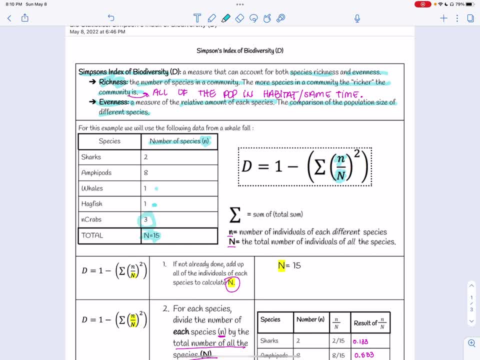 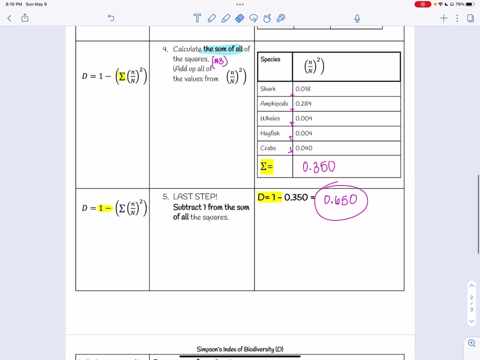 Gross. You've got a cleanup crew right there with your crabs. You've got another cleanup crew with the amphipods And two top predators there, which would be the sharks. Okay, So 0.650 from that example: The diversity. 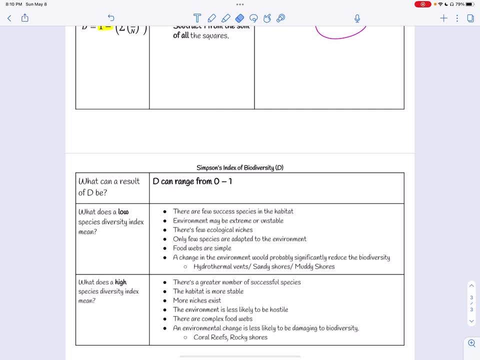 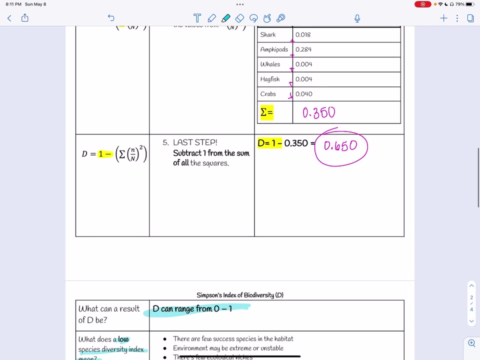 The diversity can range from 0 to 1.. Where having a low- so being like I don't know- around a 0 range would mean that you're going to have low biodiversity And so obviously, having in the higher range- and this is kind of like higher, like higher middle. 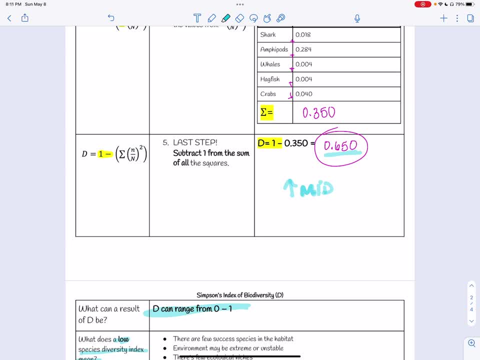 You're going to have more diversity And typically you wouldn't just execute this on just one habitat. You would probably do it for two And then compare what habitat is more biodiverse than another. Or it might say, like a student concluded, that you know, the rocky shore was more biodiverse than the estuary. 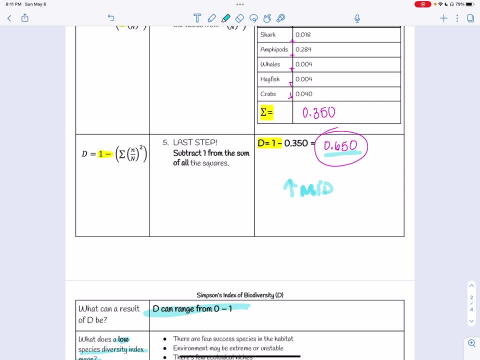 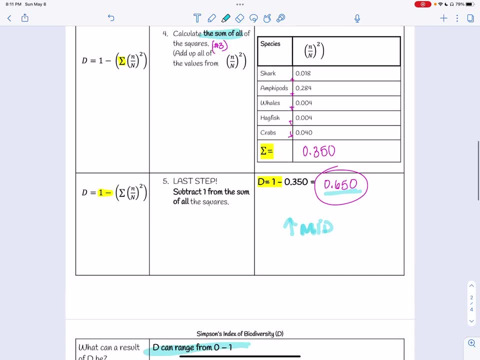 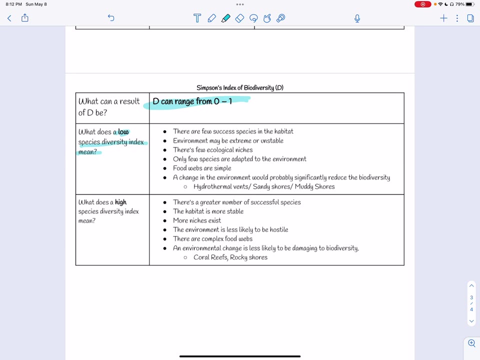 Do you agree with this? Or, yeah, assess the student's findings essentially, And so then you might need to go do this calculated value for both of them to make that assessment, And they did see that on their paper too, actually. 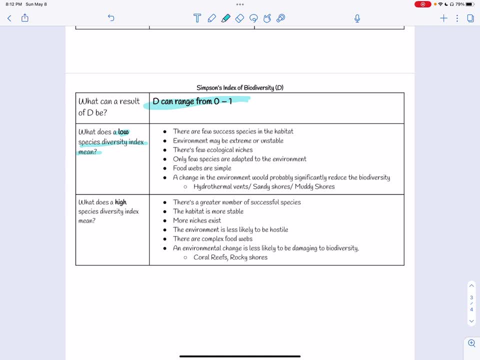 All right. So if it's a low biodiversity or it's a low value, then we're going to assume that there's very few successful species in the habitat, And that should say successful. Okay, So we're doing it on the same. The environment could be extreme or unstable. 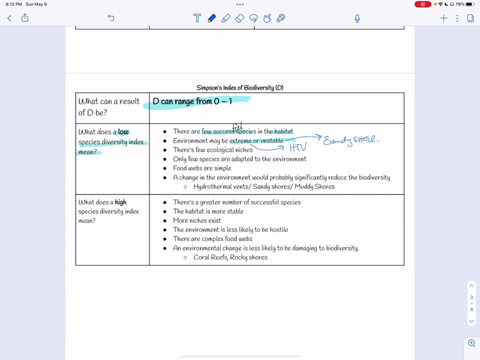 Remember, extreme is like your hydrothermal vent, But hydrothermal vents are always extreme, so they are also stable. Because they're always extreme, there's gonna be few niches or few roles for organisms to occupy. only few species would be adapted to be in that environment. perhaps for this one. we know that the 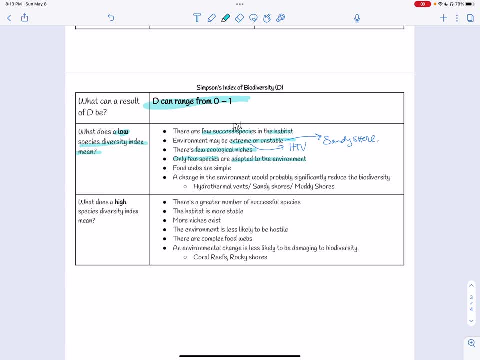 a whale fall is not going to be a habitat. that's going to be something that's consistent. it's not going to be there for a while. it's literally only there for as long as the biomass of the whale is there, and then, you know, the whale fall itself will go through succession, and at each different 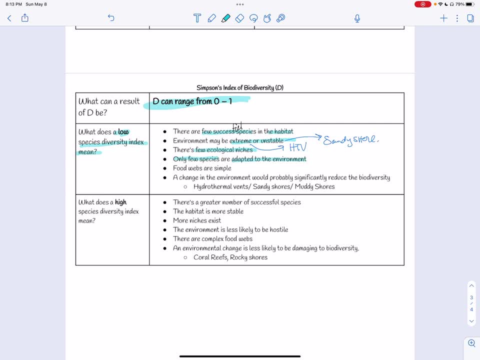 succession stage. you're gonna have organisms coming and going. I can also assume the food webs are going to be simple and because there's not many species there and there's not many of any species there, there's not many different species and within those species there's not. 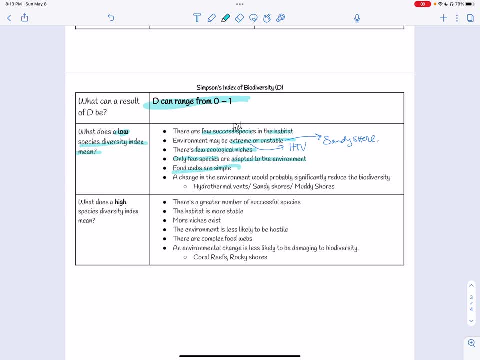 a lot of them anyways, then we can assume that there's probably unique situations there and if there were going to be any kind of environmental change, it would be hard for them to adapt to that. that would most likely bring down the biodiversity. so changing the environment would probably reduce the biodiversity. so hydrothermal vents, sandy. 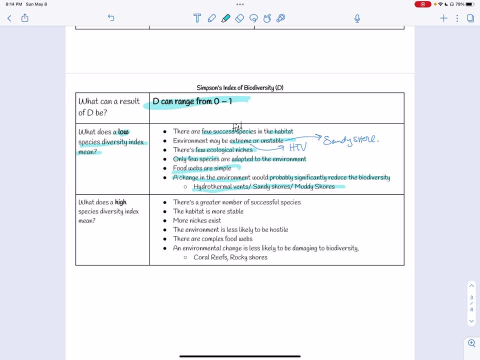 shores, even muddy shores. remember muddy shores are anoxic. oftentimes they can be acidic as well. you have a lot of noxious gases there, a lot of sulfur, because of all the anaerobic respiration organisms who live in the muddy shore, for example, your mangrove. they're gonna have to be able to adapt to that anoxic soil by sticking. 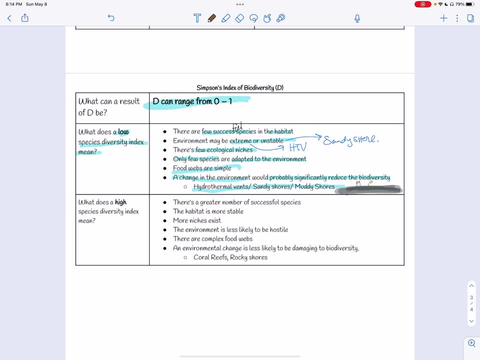 up some nematophores out of there, like those little snorkels, so that they are able to adapt to that environment. if it's a high biodiversity index, so gonna be. you know, the higher range of like 0.5, and that would even be in the middle, but if it's higher, obviously. 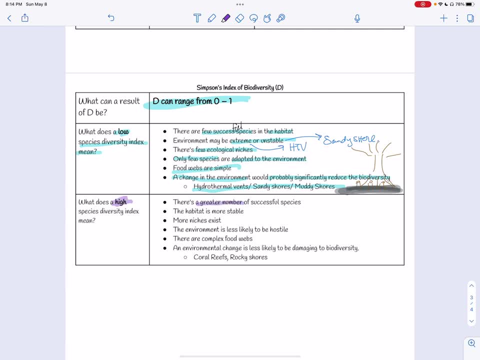 the highest would be in the nines. we know there's a greater number of sexual speed successful species. the habitat is stable, so organisms are able to live there and adapt to it because they're only having to adapt and live in the conditions that they're facing all the time. more niches or more. 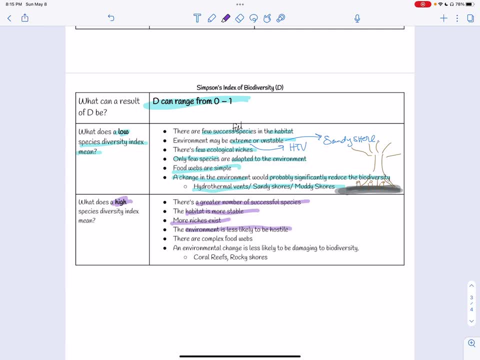 roles will exist and the environment is less likely to be hostile. um, there's probably going to be ample amount of sunlight, perhaps. um a sustainable amount of food. the oxygen there is- is always going to be available. um, it won't be under really high pressure, it won't. 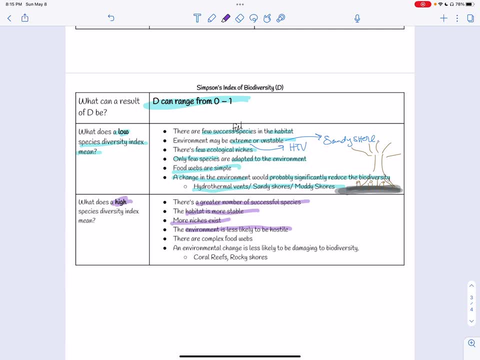 be acidic, the ph won't fluctuate like crazy. so, um you know, like in an estuary or even in like a rocky shore tide pool, you can have high fluctuating abiotic conditions. um the complex or the food webs are going to be complex. the food webs are going to be complex, the food webs are going to be complex.